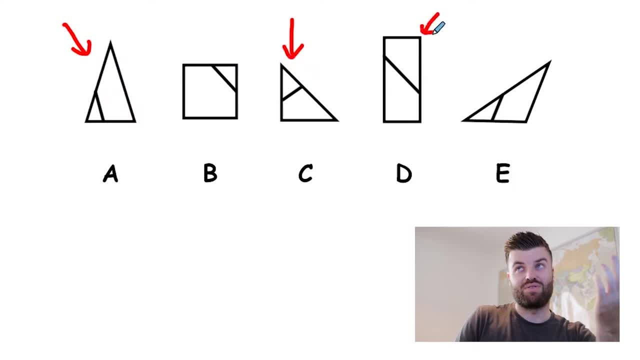 out. Could it be that it's a four-sided shape? Well, no, because the next shape is also a rectangle, So we can see straight away that the odd one out can have nothing to do with the number of sides the shape has, because we don't have one. 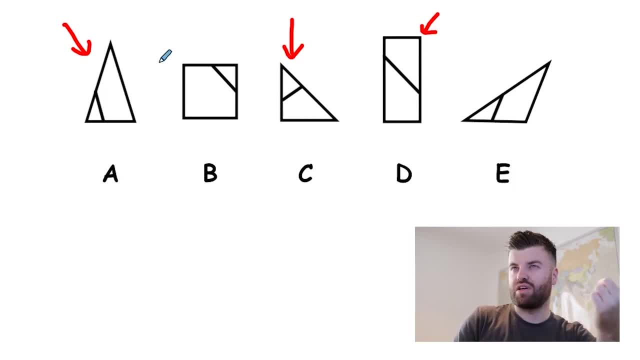 That's different to the other four. So let's move on and take another look. There's something to do with the line here. inside of the shape, They all have a line, so it can't be the fact that there's one line or two. This one here comes across and it makes a triangle inside. Let's see what the 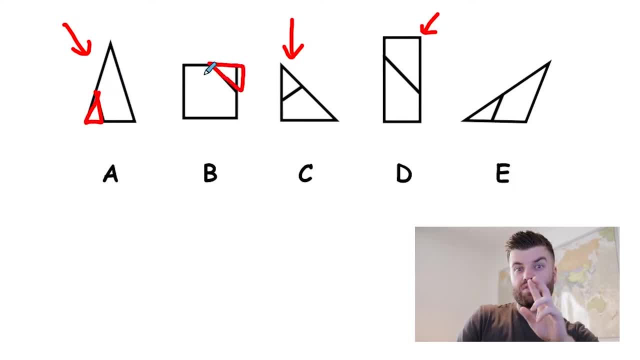 others do. This one comes across, makes another triangle, so that's two the same. This one here comes across and makes a triangle, That's three the same. This is looking promising because, remember, we want four the same and one different. The next one. 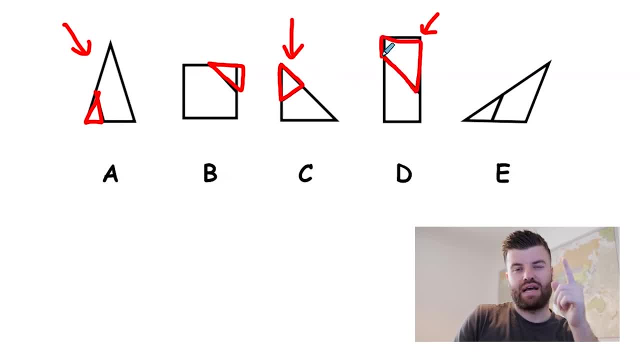 doesn't make a triangle. Now, it could be that this is the odd one out. If the final shape makes a triangle with the line across the shape, then we know we've found our answer. Let's have a look, and it does So. E makes a triangle with the line going across. We have one, two, three, four, small. 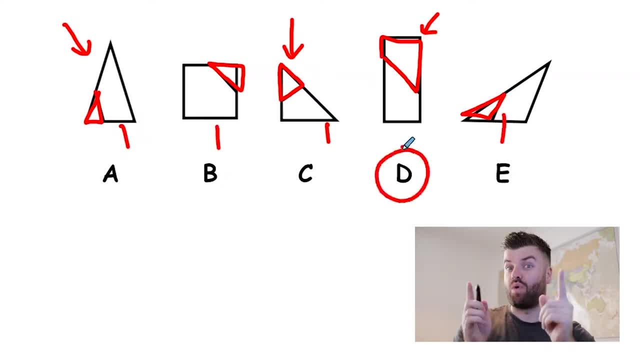 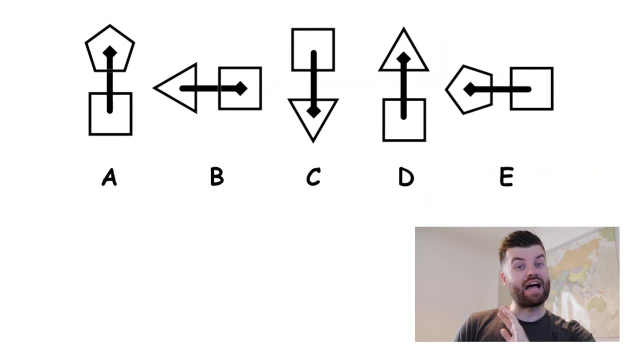 triangles inside of the shape. Therefore, D is the odd one out, So let's take a look at another one. remembering this logic, We need one shape that's different to the other four, and those four have the same shape. So let's have a look at A. We're given a square and a pentagon, So we have a square. 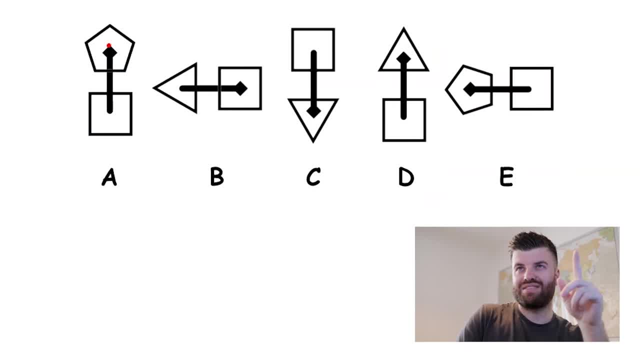 and a pentagon. There's a line joining them up and you can kind of see the head of this arrow. here is inside of the pentagon. Let's take a look at the next one. We have another square. Let's have a look at that then. Do all of these shapes have a square? Yes, yes and yes. So it's nothing to do. 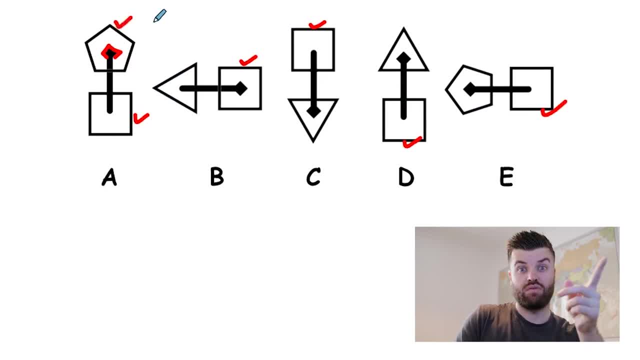 with having a square. Let's look at the second shape. We have a pentagon, a triangle, a triangle, a triangle and another pentagon. Unfortunately, that can't be the odd one out. We have two pentagons and three triangles. We must. 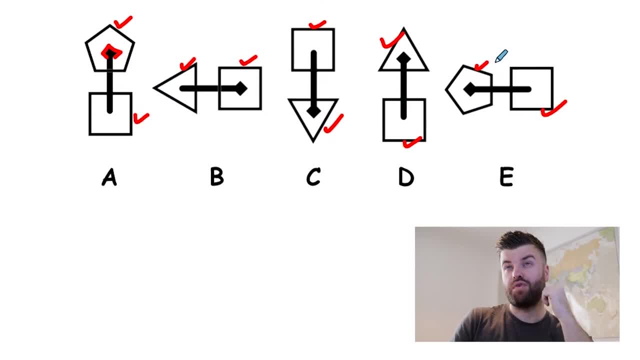 keep looking for something else where just one is different to the other four. Now, it must be something, therefore, to do with the line. So let's have a look at the line and maybe where the head of the arrow is. The head of the arrow here is in the pentagon, which means we have a blunt end in 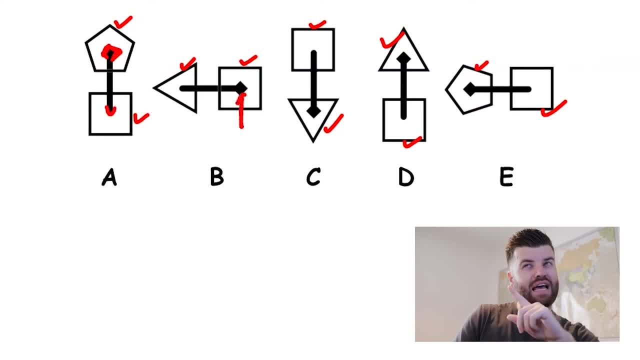 the square. Aha, here we have the head of the arrow inside of the square. Let's keep going, because these are different. somehow We can find some similarities. We might have an odd one out. already We have a blunt end in the square, The next one has the blunt end in the square and the final one 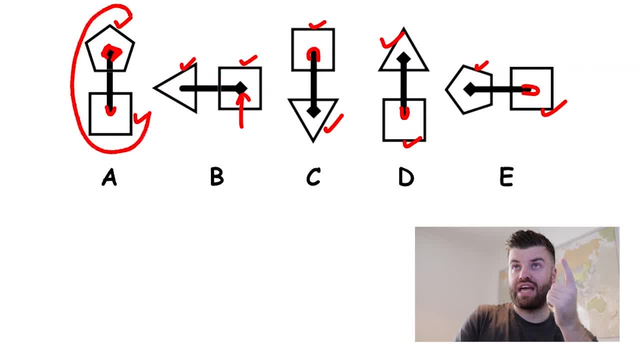 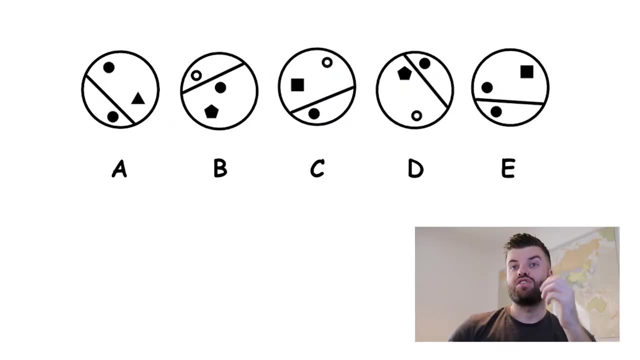 also has a blunt end in the square. So we have four shapes here with the blunt end of the arrow in the square and one shape that's different. This must be our odd one out. One shape that's different, four that are the same. somehow We'd circle B and we move on. So here we have a third odd one. 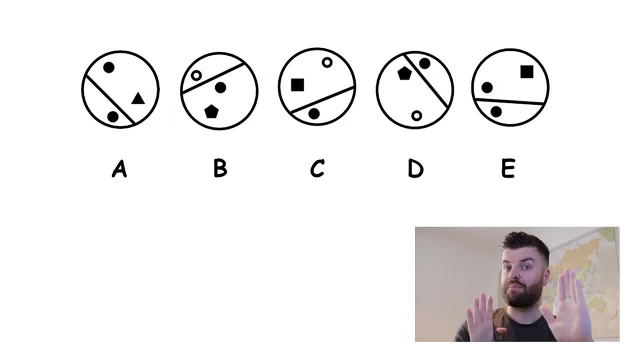 out question, and what I want you to do is have a go yourself. So remember, you are looking for an odd one out. You need to be able to justify how the other four are the same and your shape is the only one that's different in that respect. So I'd like you to pause the video and have a go. 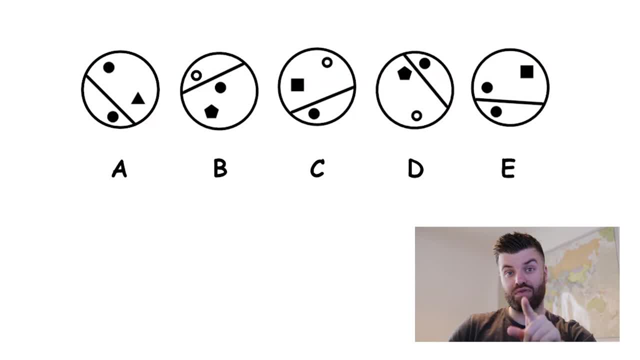 for yourself. Leave us a comment down below if you've got an answer and we'll go through it together in a minute. So hopefully you've got an answer. now We can have a look together and see how you did. We are given five shapes. again, There are five circles. 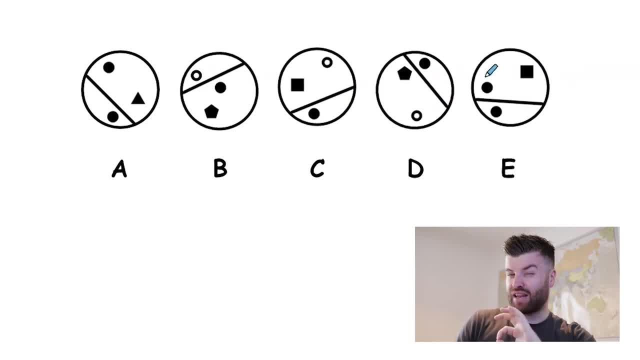 so it can't be anything to do with the circle. Each circle has a line, so it can't be anything to do with the line, because they're all the same. Let's start by having a look at what's different between these shapes, And I can see straight away that we have two black circles here. 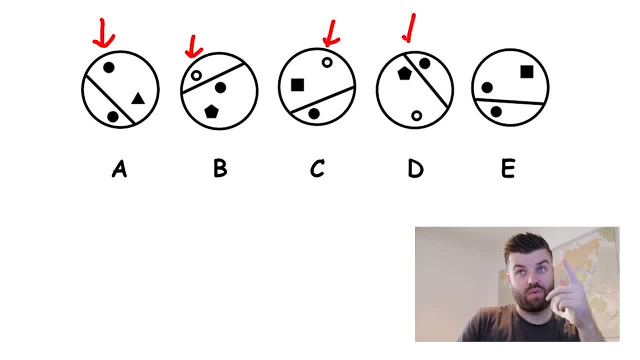 one white circle, one white circle, another white circle. So you might be thinking it must be A, because the rest have white circles. However, E does not have a white circle, So we cannot say that A or E are the odd one out, because they share that. 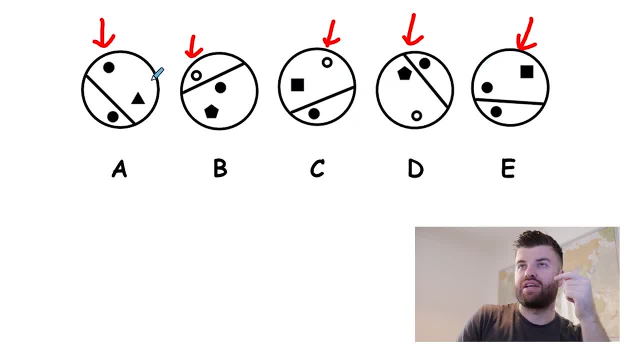 It's quite common. They both have two black circles. Let's have another look. We have a triangle, We have a pentagon, a square. They're all different. A pentagon again and a square again. Aha, At this point you might think: well, A is the only shape with a triangle.